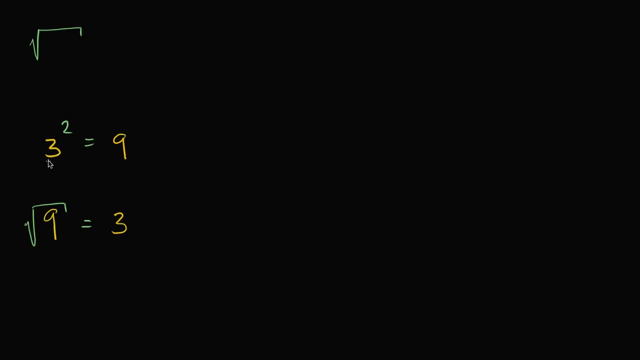 And well, that's going to be three And three squared is equal to nine. I can do that again. I can do that many times. I can write four. four squared is equal to sixteen. Well, what's the square root of sixteen going to be? 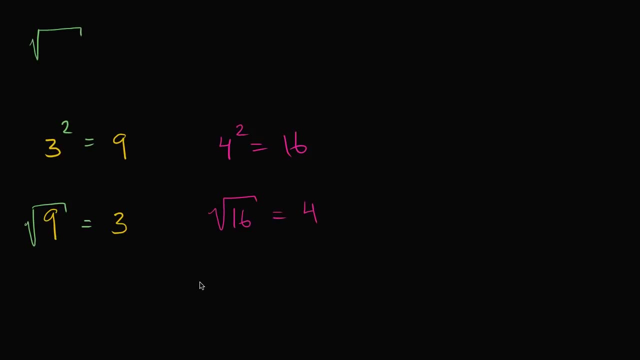 Well, it's going to be equal to. it's going to be equal to four. Let me do it again, And actually let me start with the square root. What is the square root of twenty-five going to be? Well, this is the number that times itself is going to be equal to twenty-five. 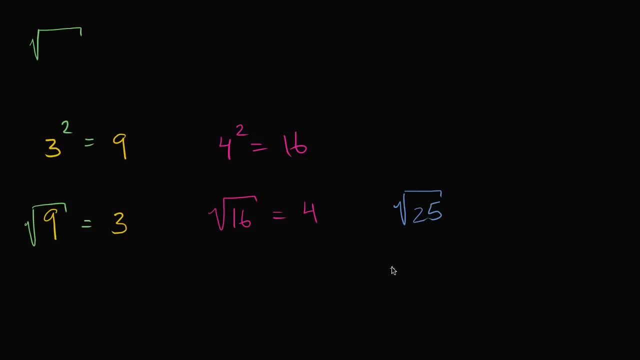 or the number where, if I were to square it, I'd get to twenty-five. Well, what number is that? Well, that's going to be equal to five. Why? Because we know that five squared is equal to five squared is equal to twenty-five. 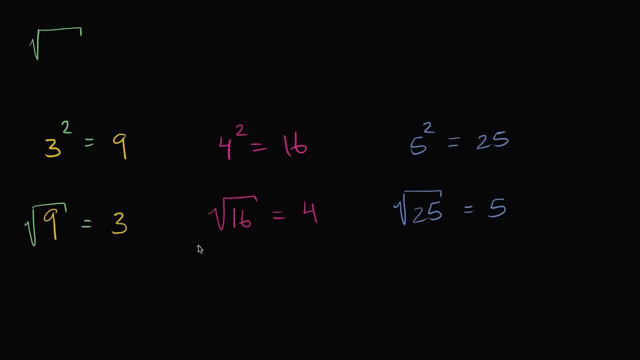 Now I know that there's a nagging feeling that some of you might be having, because if I were to take, if I were to take negative three and square it, I would also get positive nine. And the same thing if I were to take negative four and I were to square the whole thing. 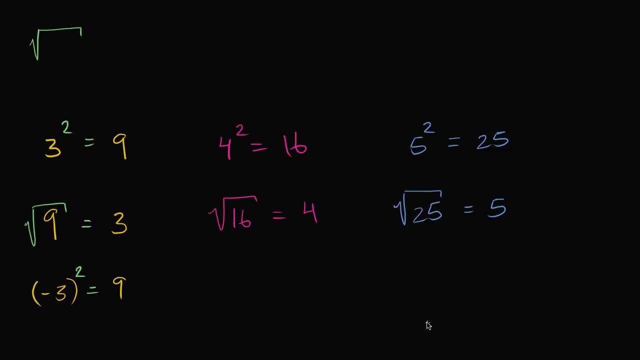 I would also get positive sixteen or negative five, and if I were to square it, I would also get positive twenty-five. So why couldn't this thing right over here? why can't this square root be positive three or negative three? Well, depending on who you talk to, that's actually a reasonable thing to think about. 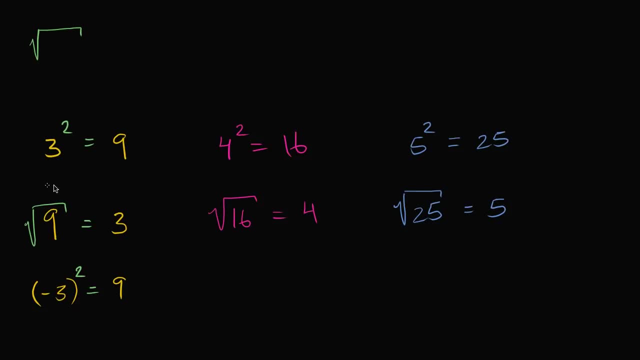 But when you see a radical symbol like this, people usually call this the principle, Principle root, Principle, root, Principle, Principle, square root, Square root. And another way to think about it. it's the positive. This is going to be the positive square root. 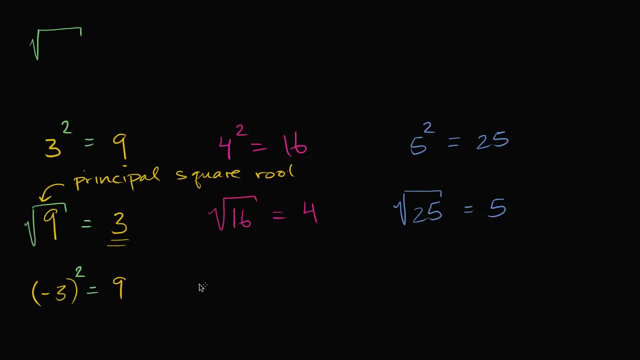 If someone wants the negative square root of nine, they might say something like this: They might say the negative. Let me scroll up a little bit. They might say something like the negative square root of nine. Well, that's going to be equal to negative three. 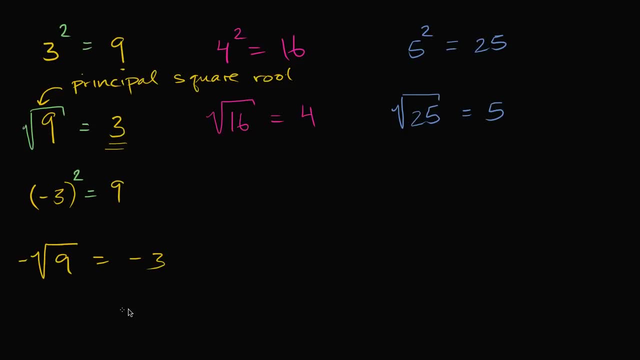 And what's interesting about this is well, if you square both sides of this, of this equation, if you were to square both sides of this equation, what do you get? Well, negative. anything negative squared becomes a positive. And then the square root of nine squared.